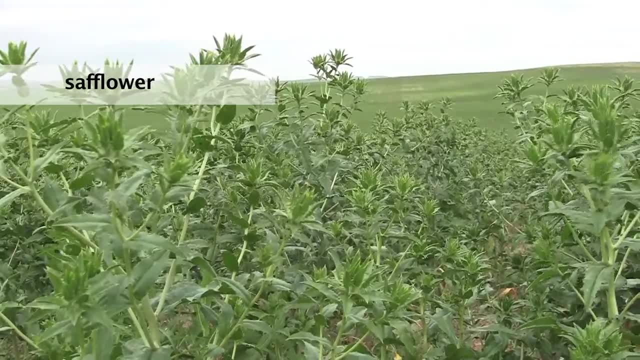 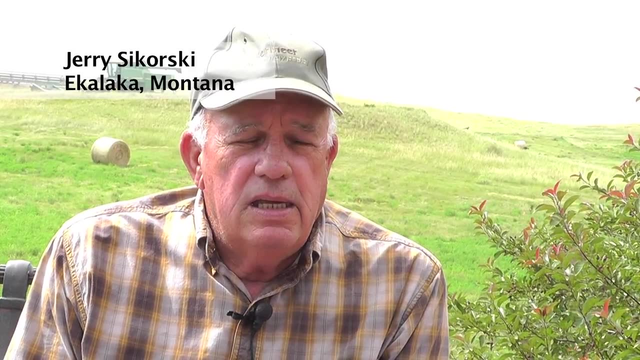 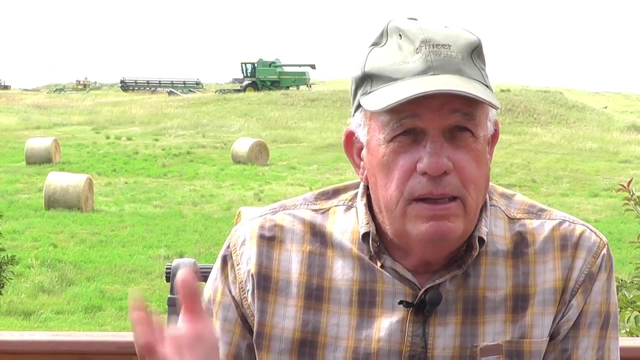 benefits. For example, plants that have a longer rooting system can scavenge nitrogen from deeper areas of the soil profile. That opens a way for nutrients to come up. Other benefits of diverse crop rotations include spreading the production risk, such as weather and market. 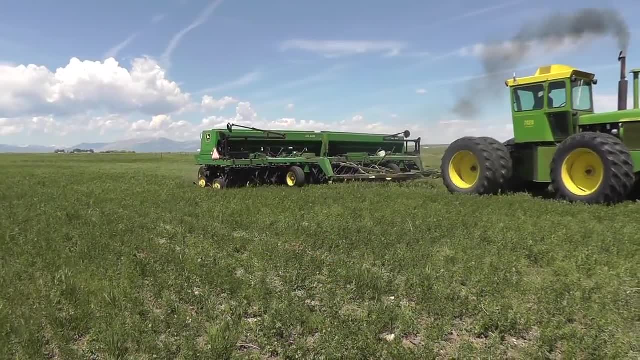 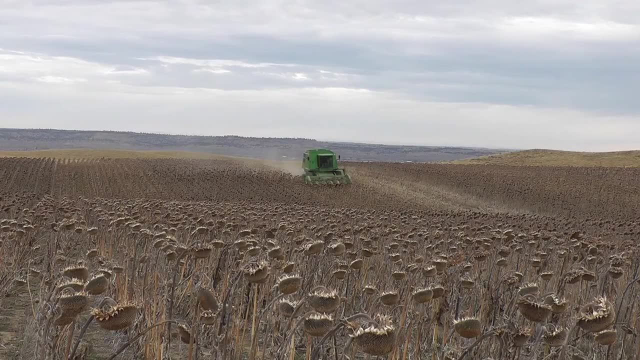 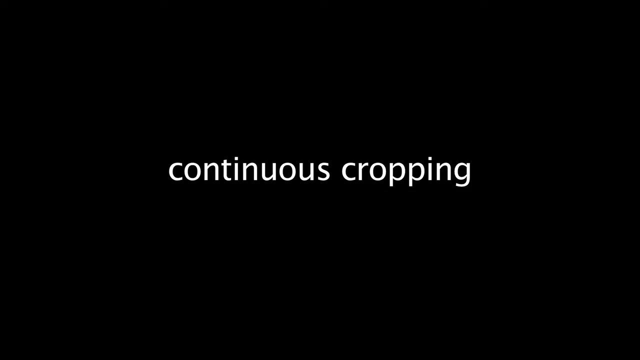 conditions and spreading the workload, such as having crops with different planting and harvesting dates. In other words, diverse crop rotations are designed so that the crops complement each other. Crop rotations are a well-established conservation practice in many parts of Montana. If you have been practicing no-till, you are already benefiting soil. 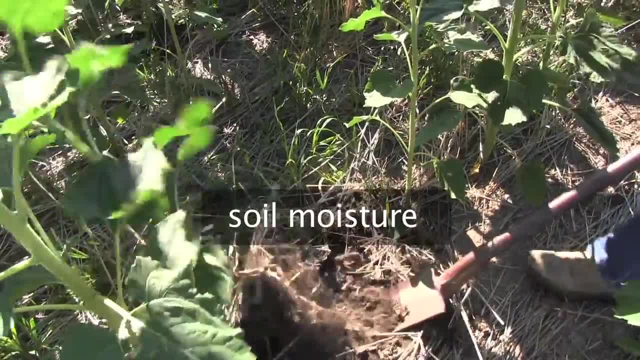 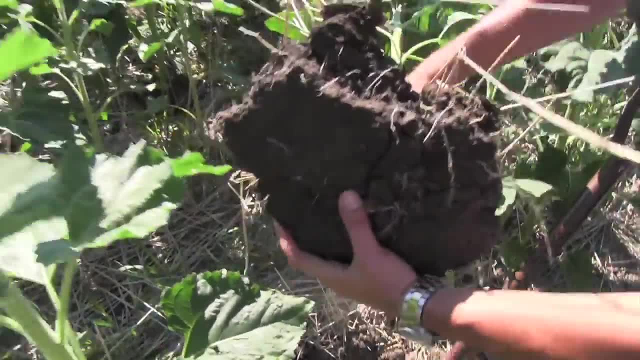 water holding capacity in several ways. Because you are not breaking up the structure of the soil each year with tillage, the soil pores remain intact and are able to improve water infiltration into the soil and maintain soil water holding capacity. You also avoid exposing the moist soil to surface. 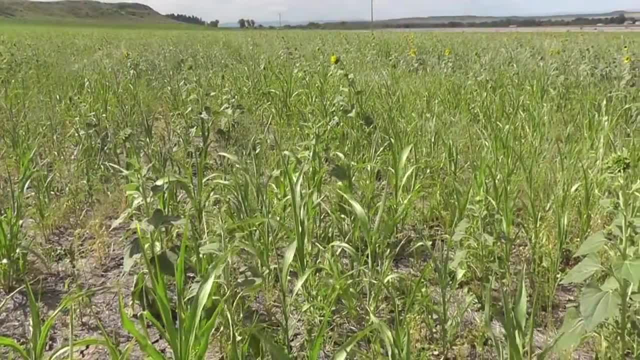 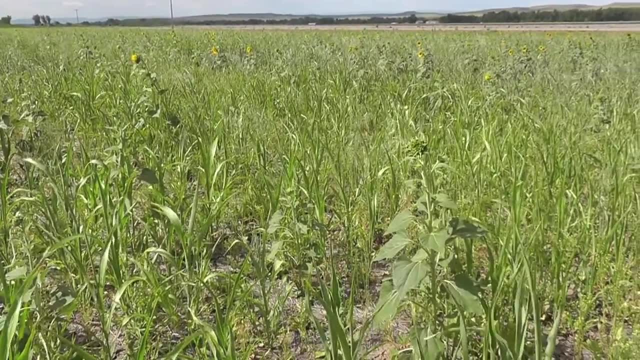 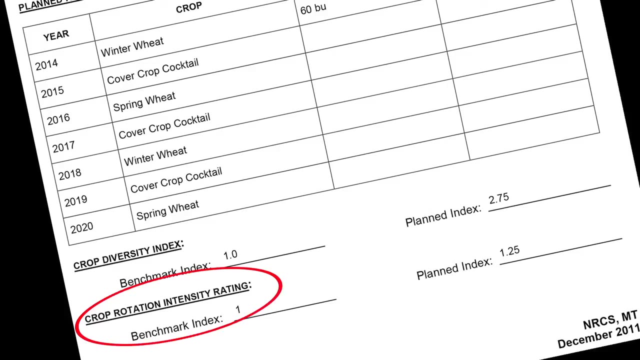 conditions that dry out water you already had in the soil. Adding various crops and keeping the ground covered will add more organic matter and therefore increase the maximum moisture capacity of your soil. When designing a crop rotation, you want to be careful you are keeping the intensity of the rotation in the forefront of your mind. 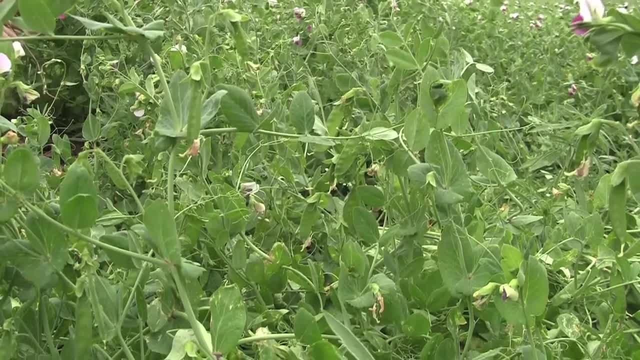 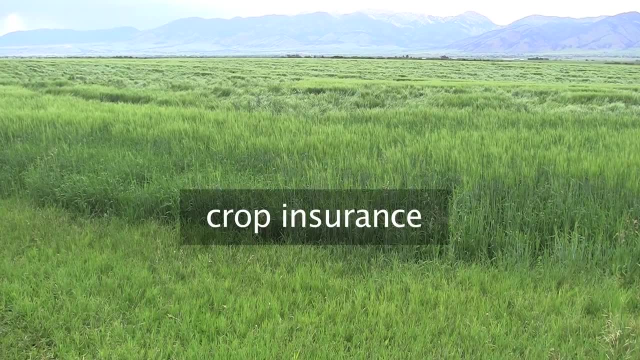 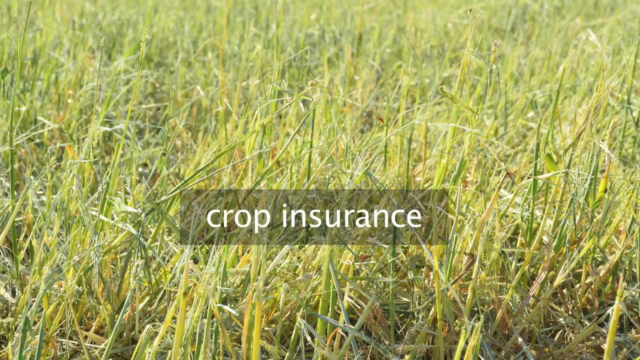 Crop intensity balances warm season and cool season crops. You want to match the water use intensity of your crop rotation to the native range surrounding you. A second concern with transitioning to continuous cropping is crop insurance and the implications changing your system may have for that. 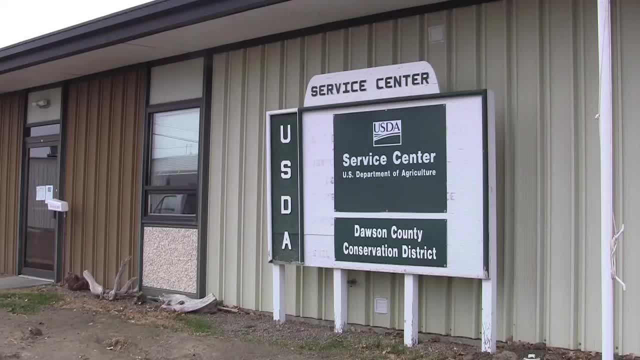 For this issue. each farmer should discuss the proposed change with the appropriate USDA agency. Crop monthly is a прошisor provision. Calculating negotiated losses can be recommended and were수 rightly listed using the 번's date, The carbon to nitrogen ratio on. 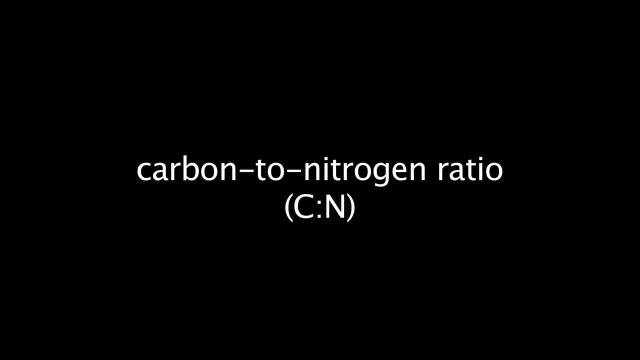 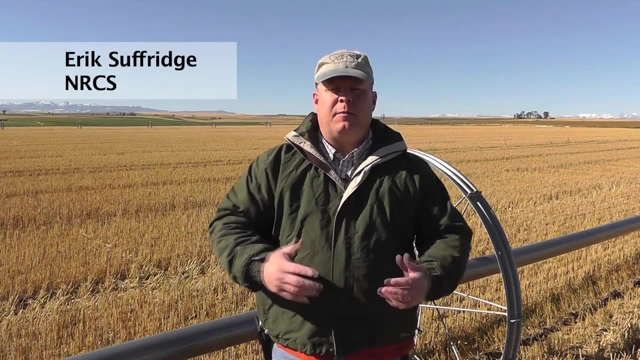 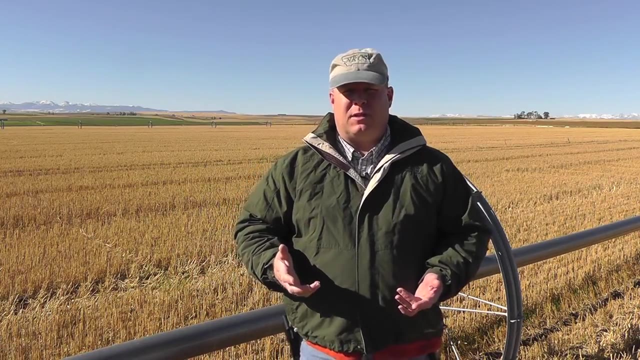 the surface and in the soil is important during the entire crop rotation. The carbon to nitrogen ratio is the ratio of the amount of carbon per the amount of nitrogen. The carbon to nitrogen ratio is important because it helps to control preached The availability of the nitrogen that's in the soil. microorganisms in the soil use the 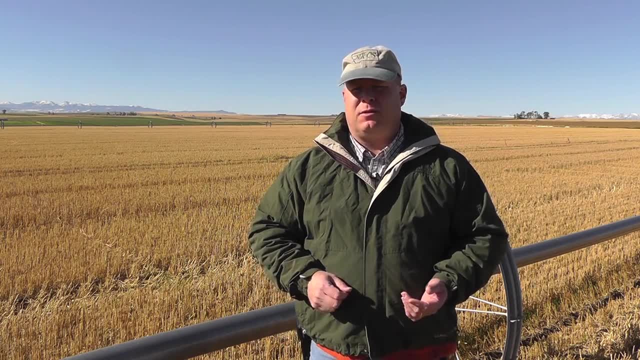 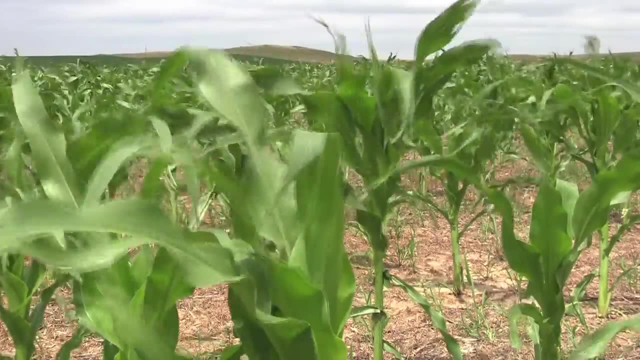 nitrogen is fuel to break down the carbon in the plant residues. What this means to you, the farmer, is that the carbon-to-nitrogen ratio controls how well and how much of the nitrogen in the soil is available to your crop If the carbon-to-nitrogen ratio is too high.